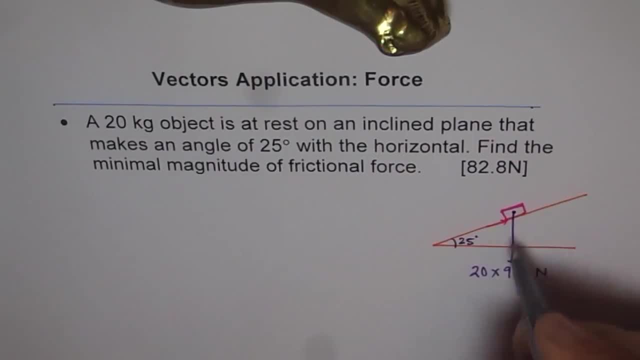 exert in the downward direction. Now, because of this force which is acting on this object, the body should move, But it is not moving, since there is an equivalent opposite force there which is keeping the system in equilibrium. right Now, let's work out how much that force is To find that we need. 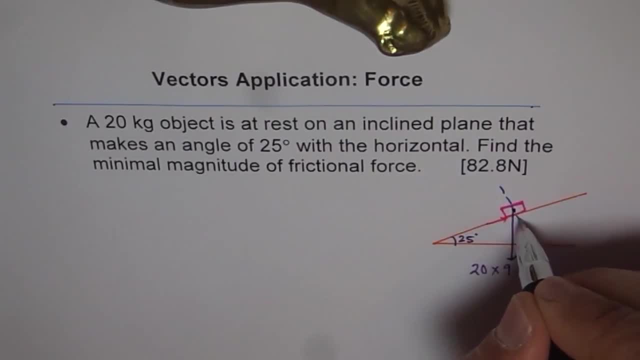 to resolve this force into its components. So we'll resolve this force into two components: one which is trying to push it downwards right And the one which is pushing at the surface right Now. if this angle is 25, then this angle is also 25 degrees. Now, as you can see, from here we can complete our 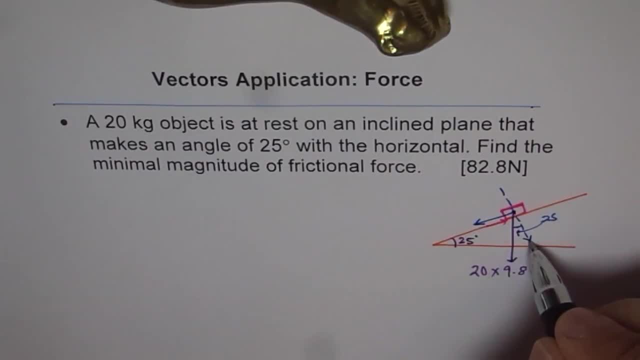 vector diagram which says: this is one force. Do you see that one force And that is the other force. So the combination of these two forces should be equal to 20 times 9.8.. So let me draw them separately here. So what I'm trying to show here is that is the. 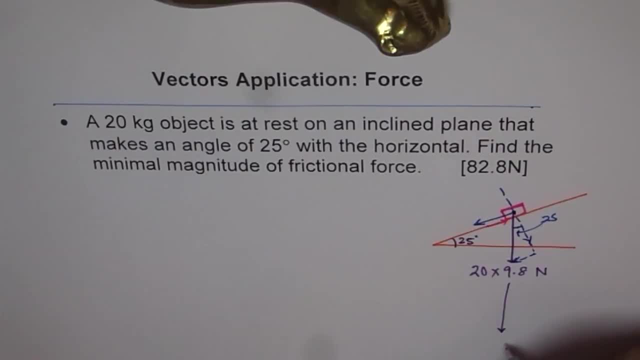 downward force And this actually is exiting a force which is normal to the surface, which is kind of here right And along the surface downwards, like this. So these are the two forces it can be resolved into right. So we have a force which is 20 times 9.8.. 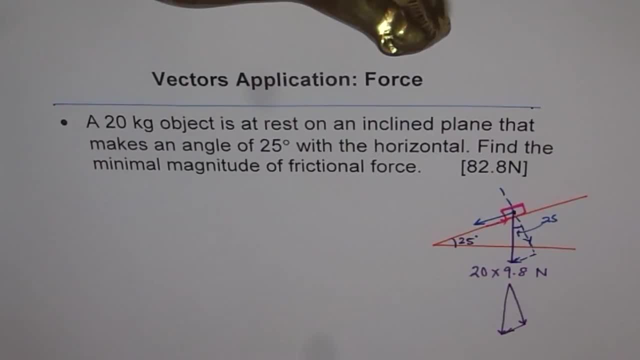 So let me multiply 20 times 9.8.. And we get a value of 196.. So this force in this direction is 196 newtons. right Now we need to find what is the component along the plane. So component along the plane is this angle which we have here is: 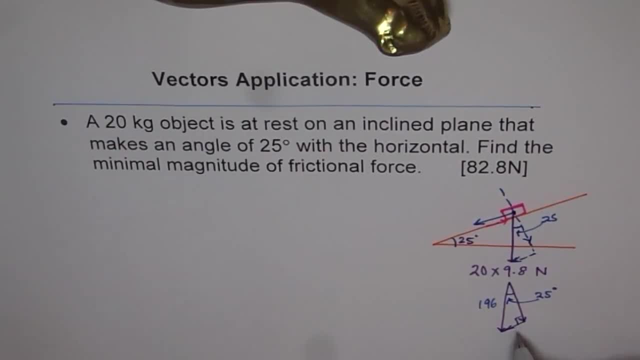 25 degrees. Now this is opposite side and that is 90 degrees. So we have taken this normal to the surface. that means it is at 90 degrees to the surface. If this is at 90 degrees, then that force which is sliding force or the downward force, 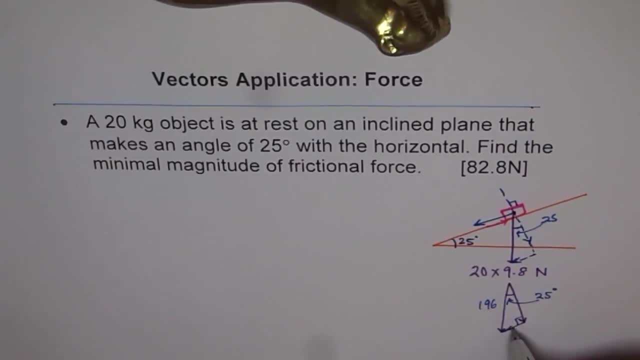 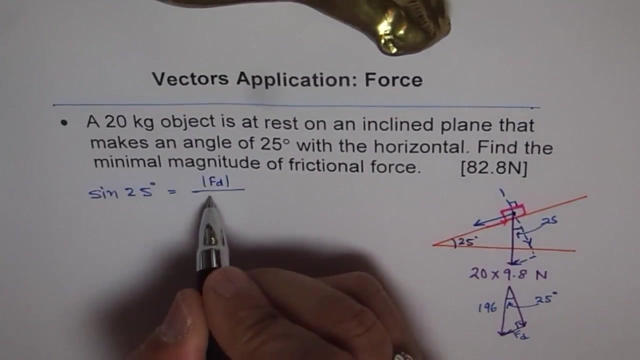 is sine theta right. It is opposite to this side, right. So we have: sine of 25 is equal to, let me call this force Sfd, the downward force, right. So sine of 25 is equal to the magnitude of force Fd over the hypotenuse, which is 196,. 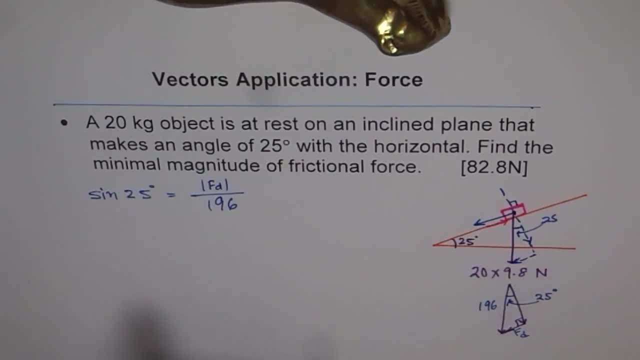 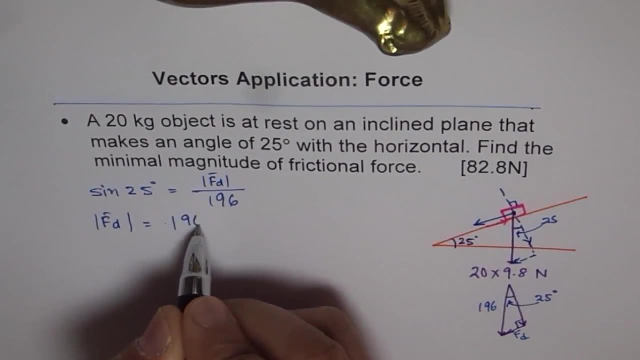 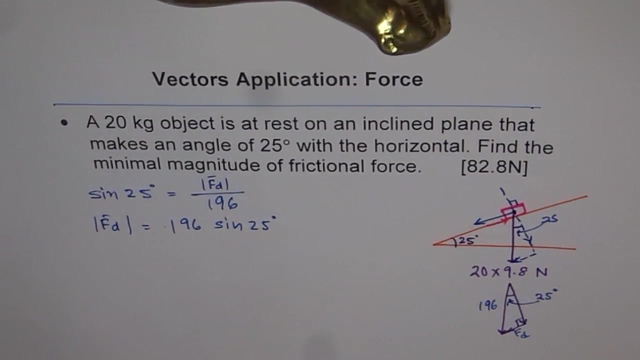 correct And therefore this downward force, which is which should slide the object, is actually equal to 196 times sine of 25 degrees right. So let's use calculator to calculate this answer: It is 196 times sine of 25 degrees right. 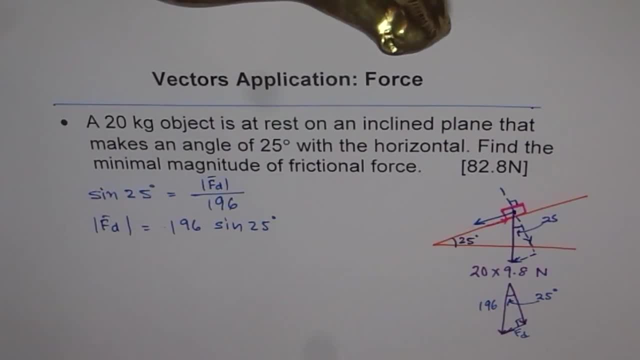 And sine of 25 degrees, we get 82.83.. So let me write this as 82.8 Newton. So that is the magnitude of force, correct? Now, because of this force, the object should slide along the slope, but it is not. 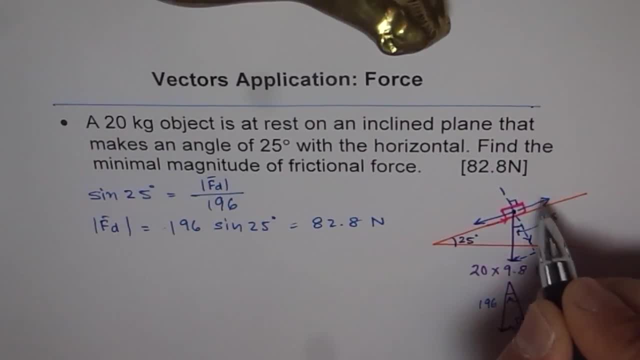 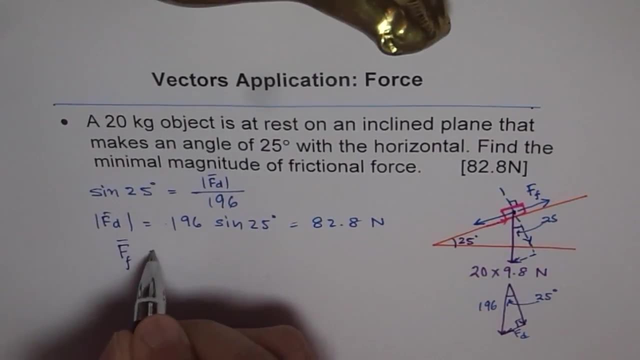 Since there is a frictional force which is acting in the opposite direction, let's call this as Ff, So frictional force, Ff. F should be equal to the magnitude of frictional force, let us say should be equal to the 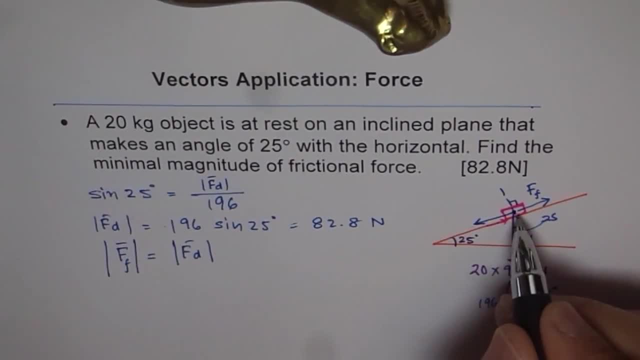 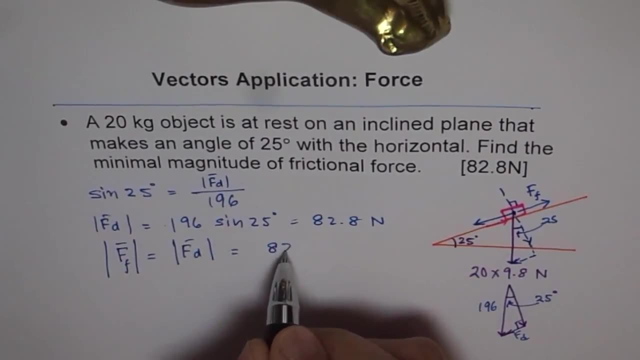 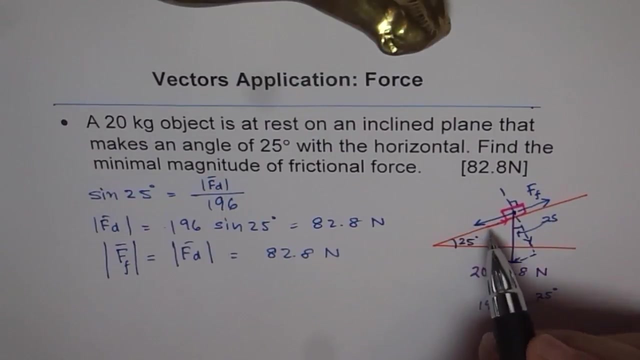 magnitude of downward force to keep it in place, And it should be in opposite direction. do you see that Now the magnitude should be equal to 82.8 Newton, since the downward force is 82.8 Newton. right, And as you can see from here, the downward force make an angle of 25 degrees with the 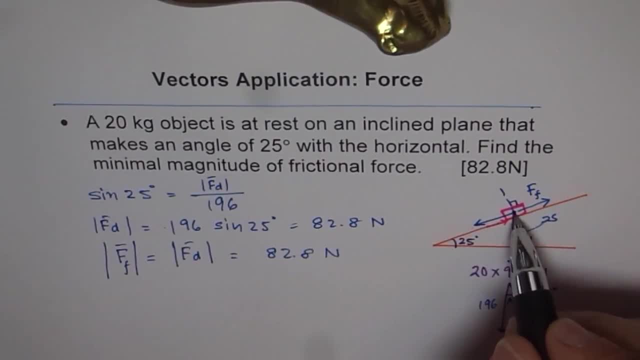 horizontal. So this one will make the angle 180 – it's in the opposite direction of 25 degrees- correct. So that is how we are going to solve this question. do you see that? So I hope you understand. 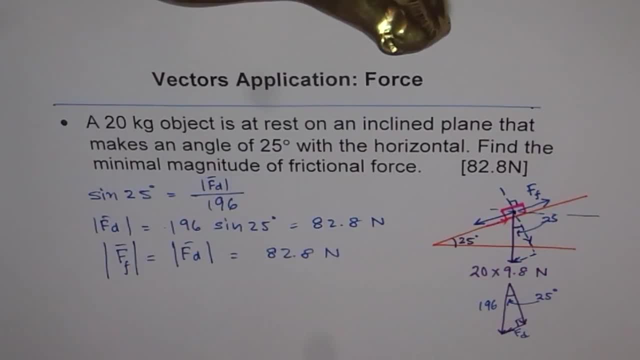 Now, the state of equilibrium is achieved if we have all the forces acting at a point and their sum is zero, right? So if we add these two forces, Since they are in the opposite direction, it should be in opposite direction, right.